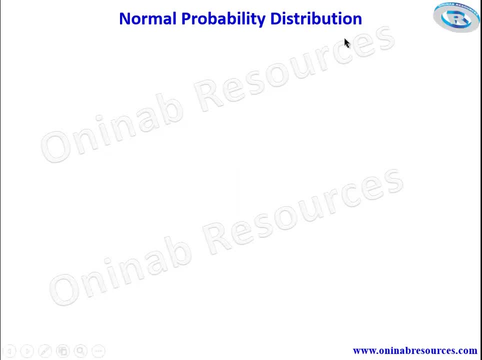 hello out there. welcome to this tutorial on normal probability distribution. so we start with introduction. basically, some random variables are best described statistically by the normal distribution function. the function is given by: p of x is equal to 1 over standard deviation. square root of 2, pi e raised to power negative half into. 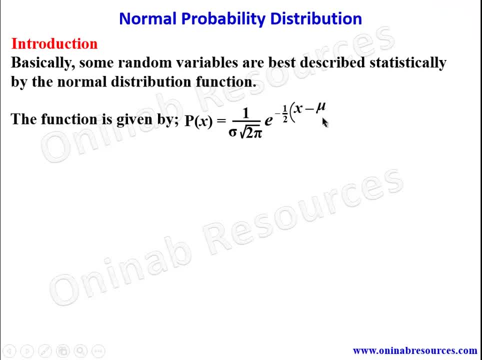 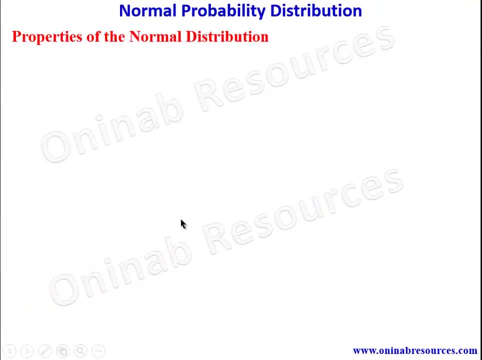 x minus the mean over the standard deviation, all to the power of 2. and we look at the properties of the normal distribution one. it depends on the mean and standard deviation b. the normal distribution curve is bell shaped and we have the diagram here. it is bell shaped with the symmetrical 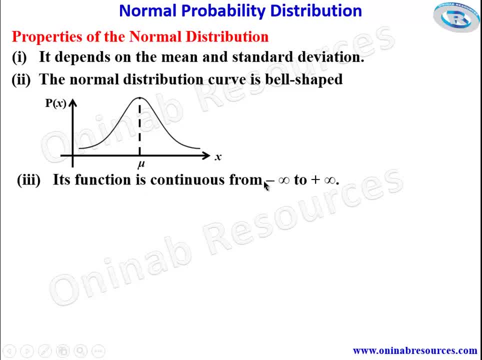 line at the mean. its function is continuous from negative infinity to positive infinity. the curve is symmetrical about the vertical line through the mean. this is the symmetrical line through the mean of the distribution and we should note that, since the normal distribution function is a probability, 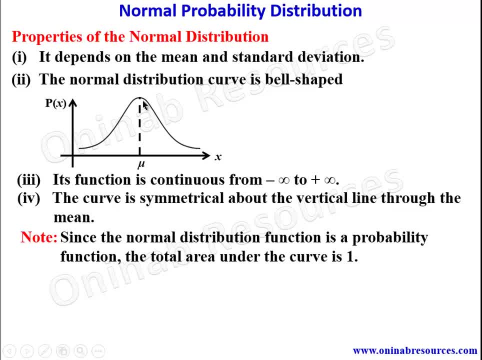 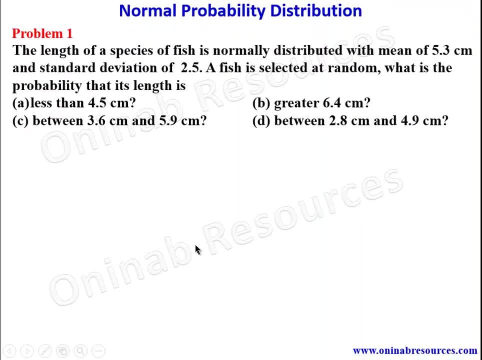 function. the total area under the curve is one, so the total area under this curve is always one. we don't go ahead to solve problems. problem one: the length of a species of fish is normally distributed with mean of 5.3 centimeters and standard division of 2.5. a fish is selected at random. what is the probability that its length is? 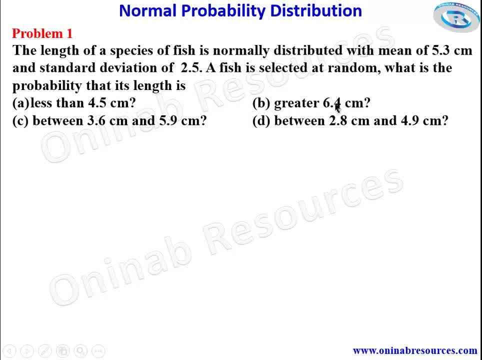 less than 4.5 centimeter, b- greater than 6.4 centimeters, c between 3.5 centimeters and 5.9 centimeters. and d- between 2.5 centimeters and 4.5 centimeters and 5.9 centimeters. so we look at the parameters we are giving. so we are giving the mean to be 5.3. 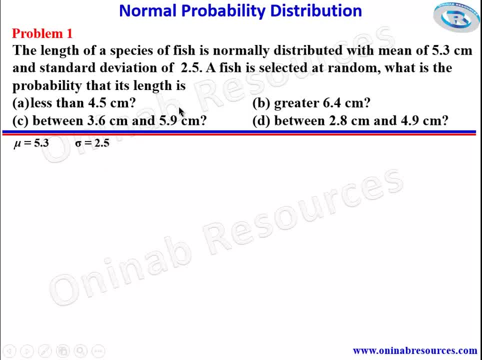 and the standard deviation to be 2.5. so, starting from a, we are looking for the probability of x less than 4.5. it is always advisable to represent this information on the probability distribution curve. so we have it here. this is the x-axis. we'll be looking at x-axis for now and the the mean is 5.3. through this, 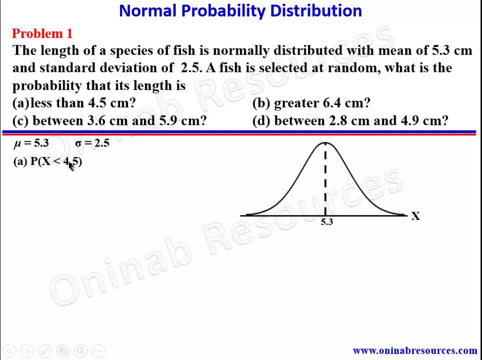 line of symmetry, and then less than 4.5 should be around this place. this is 4.5 to the left, and this is the area we are looking for less than so. we are going to convert this x value now to z, and we have to work with a formula z equal to x minus the mean over the standard deviation. 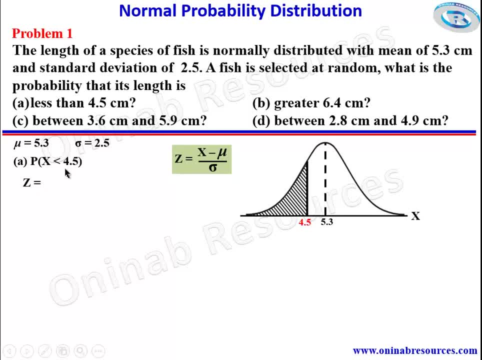 so we are going to have z to be x, which is 4.5, minus the mean, which is minus 5.3. then divided by 2.5, this would give us negative 0.32. we then bring in the z axis and the z axis is divided by 2.5. 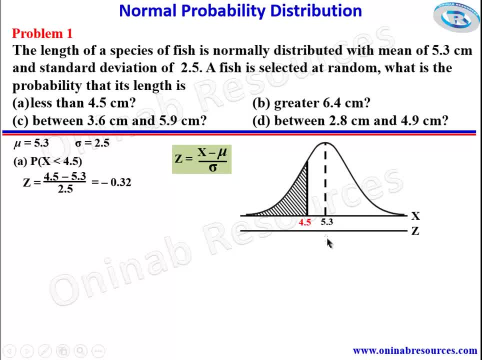 z-axis, the main point is 0 and to the left, since it is negative 0.32. we have it here: negative 0.32 is the z-score for 4.5 centimeters, so that the probability of X less than 4.5 is equal to the probability of Z less than. 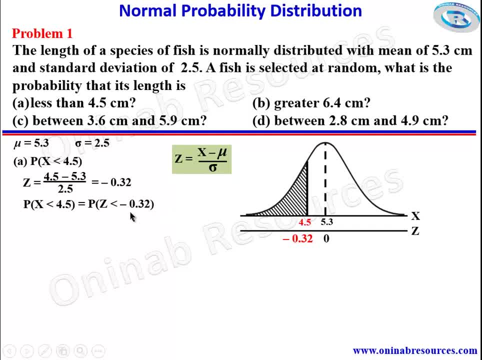 negative 0.32 and since, from here to this place, the area is 0.5, in order to get the area here now, what we'll do is the 0.5 minus this, minus this, which will give us this, and the fact that it is symmetrical. we are going to ignore the. 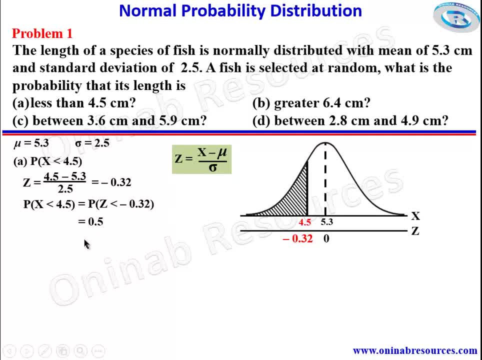 negative and return the positive value, so that the area will be 0.5 minus P of 0, less than C, less than 0.32. that is, from here to this place, is what we are going to look for, and we now take it from here to the end, which is 0.5, to give us the area of the shaded part. so 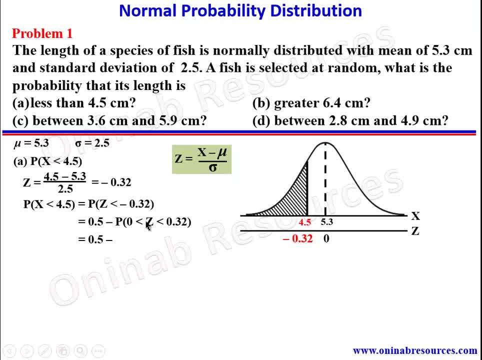 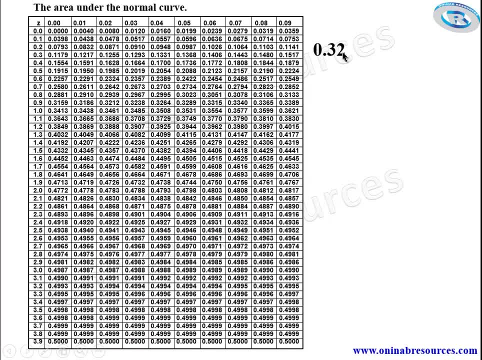 that we have 0.5 minus. this is going to be obtained from the table. so we have the table here at the 0.32 is equal to 0.3 plus 0.02. so we are going to look on to 44 Z, where we have 0.3, and to the column of zero point two, so zero. 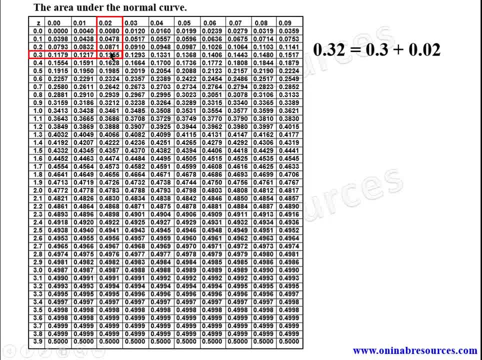 0.3. to the column of zero point. to the intersection gives the value as zero point one, two, three, five and six, two and six, two, three, five times u. and to the column of zero point two. so the intersection gives the value as 0.12. 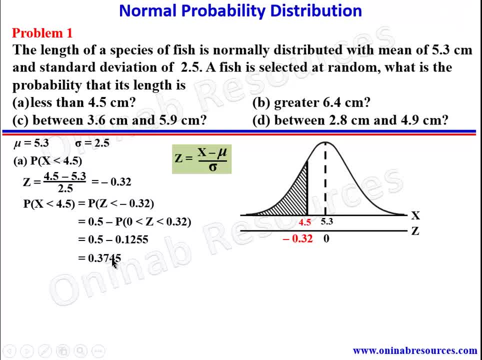 5, 5. so, simplifying this, we have 0.3745 and if you are to express this as percentage, it gives 37.45 percent. so that's all for a. we then go for b. um for b. we are true that, uh, the length is greater. 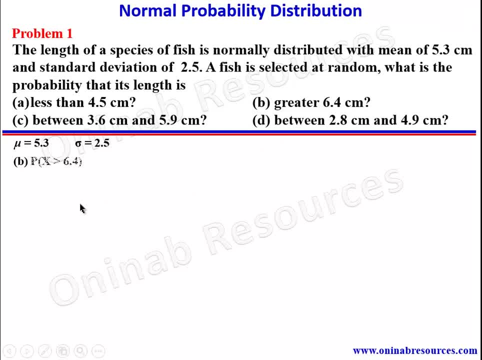 than 6.4 centimeters. so which means p of x greater than 6.4 centimeters? we still sketch this. the mean is here and 6.4 is to the right of the mean, so we have 6.4 here, the area we are looking for. 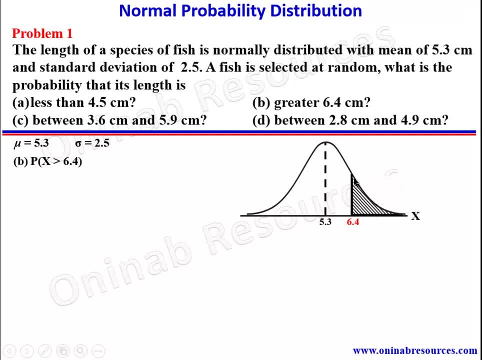 is to the right, the area of the shaded portion which will represent the probability. but before then we have to convert this to z score. so see, maintaining our formula, z is equal to 6.4 minus the mean, 5.3 over standard deviation, which is 2.5, and this gives 0.44, representing it on the z axis, the mean is 0 here and here is 0.44. 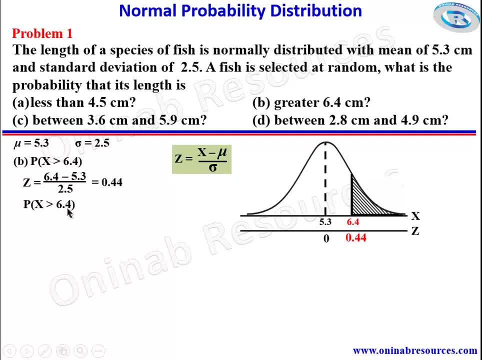 so that the probability of x greater than 6.4 is equal to the probability of z greater than 0.44. again, we look at from here to the right is 0.5. so what we do is we find the probability from the symmetrical line to 6.4 or 0.44 on the z axis. 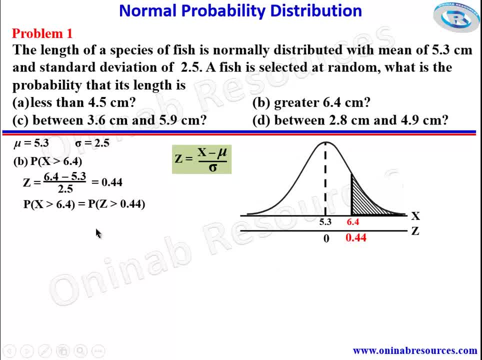 and then take it away from 0.5, so that we now have it as 0.5 minus. probability of 0 less than z less than 0.44. that will be representing the probability from this symmetrical line up to the line of the side that is shaded, so that we now have it as 0.5 minus. we go ahead again to check our table. 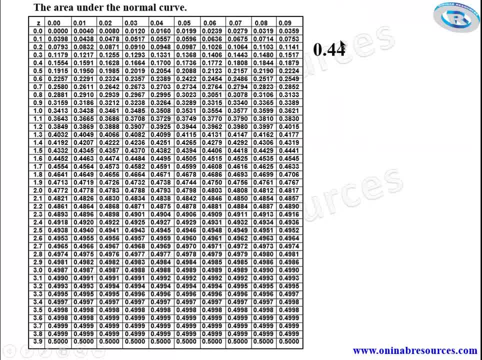 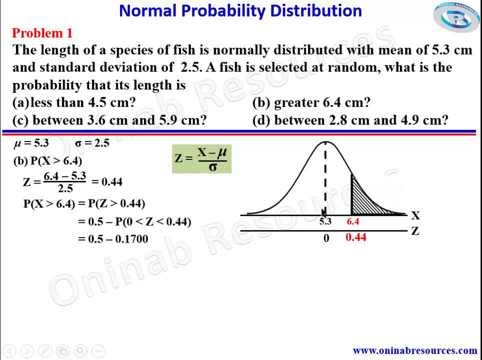 for 0.44. so if 0.44 again is the same thing as 0.4 plus 0.04, 0.4 under 0.04, and their point of intersection is 0.1700, which represents the area between this symmetrical line and this line of 0.44. 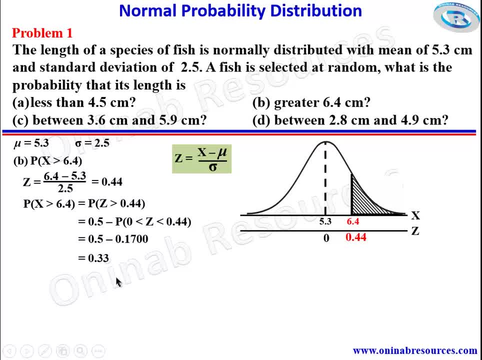 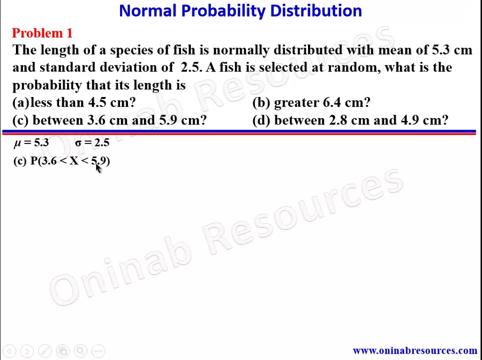 so, subtracting this, we have 0.33 and the percentage, we have it as 33 percent. and that's all for b. we then go for c. for c, we have, uh, the length between 3.6 and 5.9. what we have here is probability of 3.6, less than 5.9, um from. 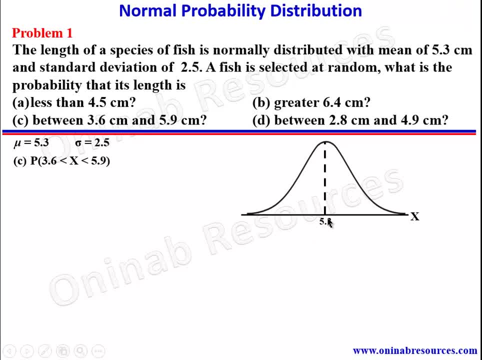 the curve. we have the mean here: 3.6 is to the left of the mean. we have the line there: 5.9 is to the right of the mean. this is the area we are looking for, which will represent a probability between 3.6 and 5.9. we then convert this to z score. 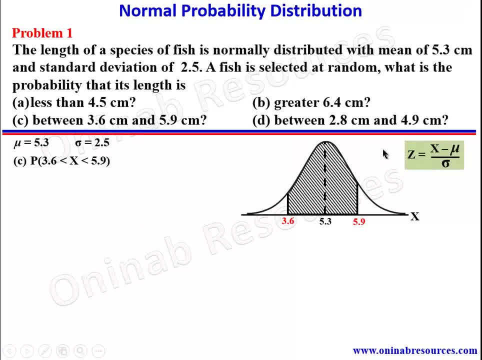 6 and 5.9 and the formula remains: z equal to x minus mean over standard deviation. we are going to have our first value of z to be 3.6 minus 5.3. divide by 2.5 and that gives negative 0.68, and for z2 we are going to have: 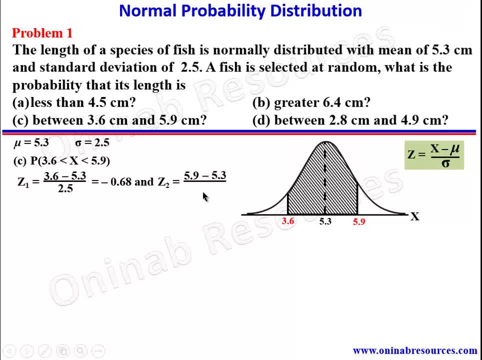 5.9 minus 5.9, 0.3 over 2.5 and that gives 0.24. so that, representing it here, our symmetrical line is c0, to the left is negative 0.68 and to the right is 0.24. so what we do is to find the area from here. 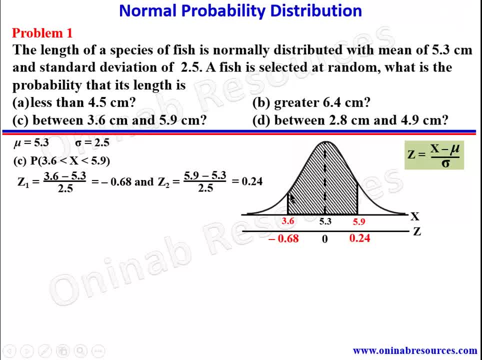 to this point and the area from here to this point and add: so this is still going to be maintained as positive, so that the probability of 3.5 less than x less than 5.9 will be the probability from negative: 0.68 less than z less than 0.24. we said we are going to find the area. 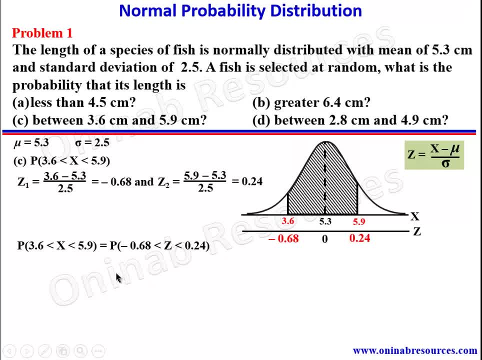 of this, find the area of this and sum them to give us the probability. so that's going to give us p of 0 less than z less than 0.68, plus probability of 0 less than z less than 0.24. so we then go ahead to find from our table. 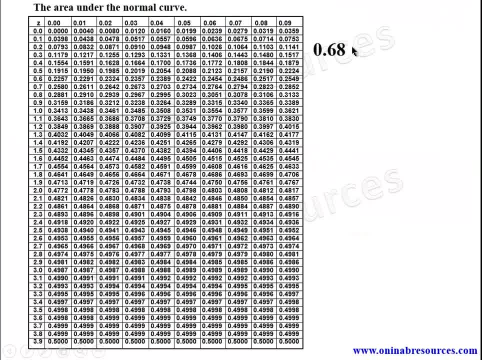 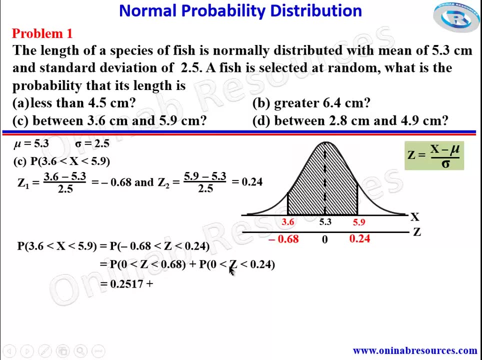 0.68. we split it again. this is 0.6 plus 0.08, 0.6, 0.6 and 0.68, 0.6 and 0.08. they are point of intersection. we have it as 0.2517, so 0.2517, then plus. we also look. 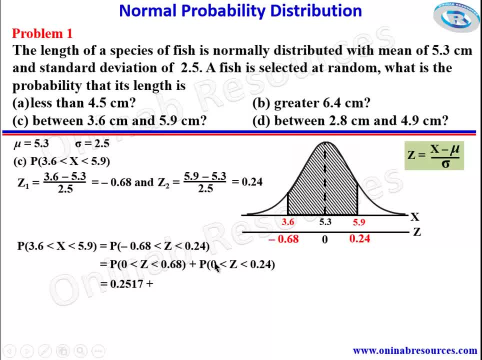 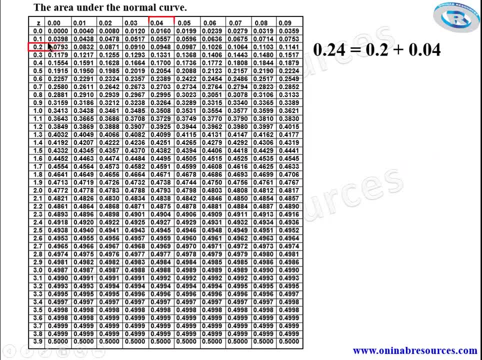 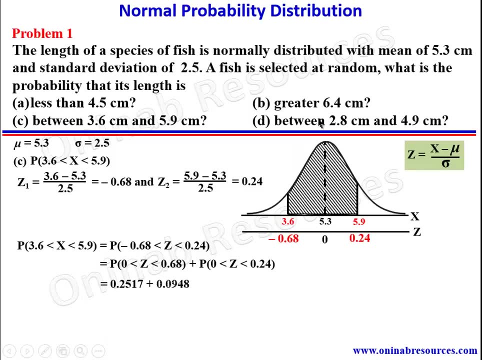 onto the table the area from 0 to 0.27. so we split again 0.2 and 0.04. so the point of intersection, which is 0.084, 0.084, 8. we then add them to give us 0.3465 and in percentage we have it as 34.65 percent. 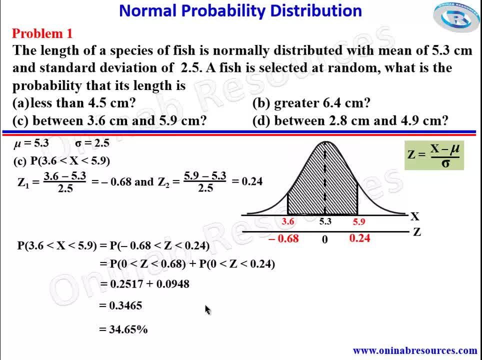 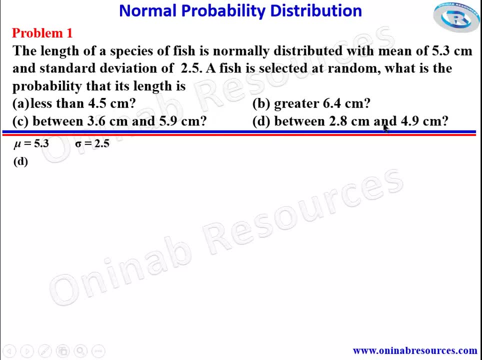 representing the probability that a fish is selected at random. its length is between 3.6 centimeters and 5.9 centimeters. puzzle for c. we then go for d. so for d, the length is between 2.8 centimeters and 5.9 centimeters. so for d, the length is between 2.8 centimeters and 5.9 centimeters. 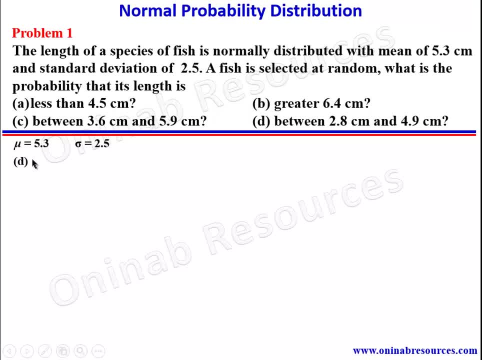 so for d, the length is between 2.8 centimeters and 5.9 centimeters, so that we now have it as p of 2.8 less and x less than 4.9, and then, sketching the curve, we have the mean to be 5.3. this is before the mean. 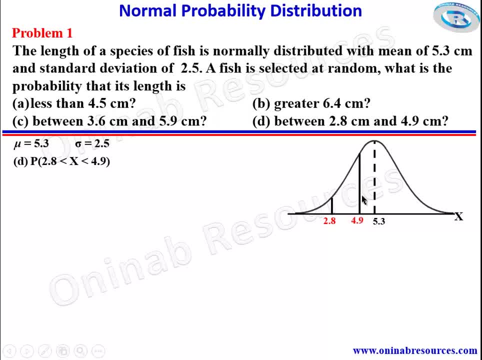 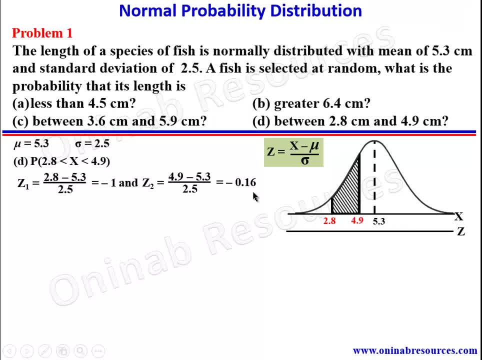 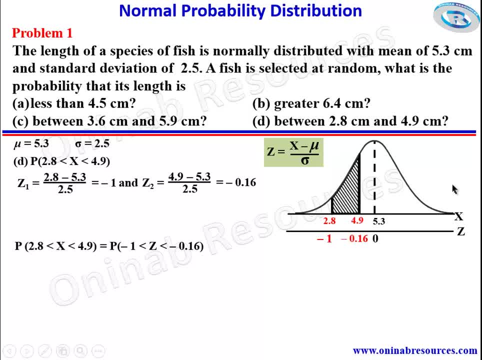 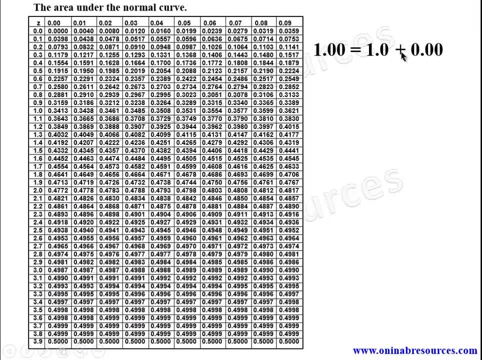 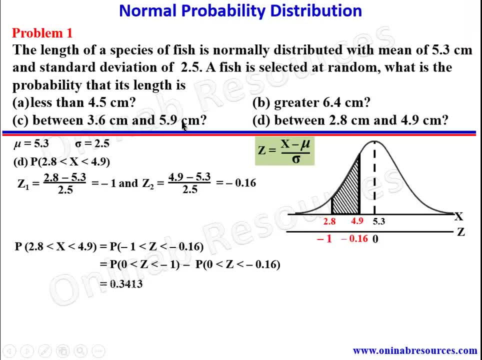 1, that's going to be 1.0 plus 0.00. this is the point here: 1.0 0.00. their point of intersection is 0.3413. then minus we look onto the table again for negative 0.16, that will give us 0.1. 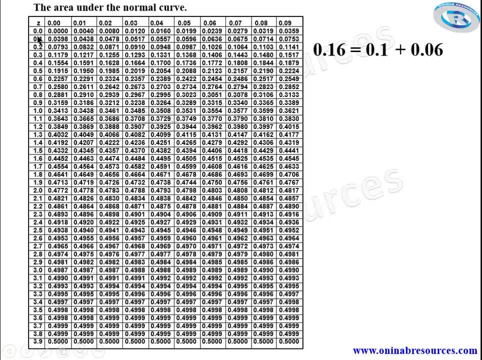 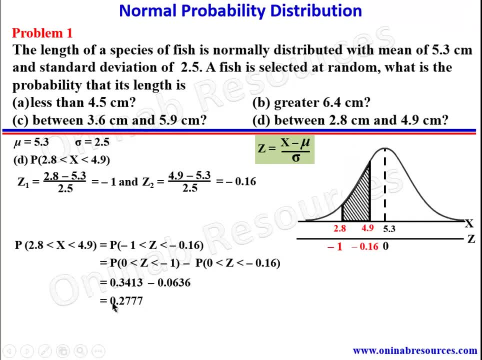 plus 0.06, 0.1 under 0.06- this is the point of intersection- which is 0.0636. so we subtract to give us 0.2777 for percentage, give us 27.77 percent, representing a probability that a fish 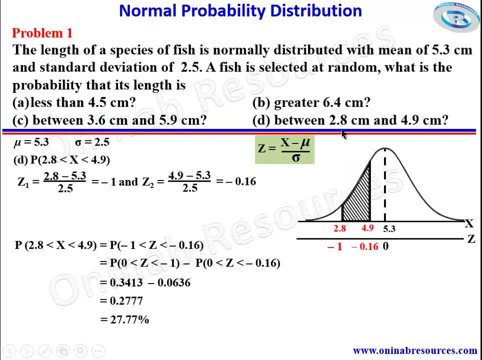 is selected at random. its length is between 2.8 centimeters and 4.9 centimeters. as the end of problem 1, this is the highest we can take in this video. see you in our next video for the second problem, on normal probability distribution. check the description section of this video on our YouTube channel. for the video, until we come your way again, goodbye.